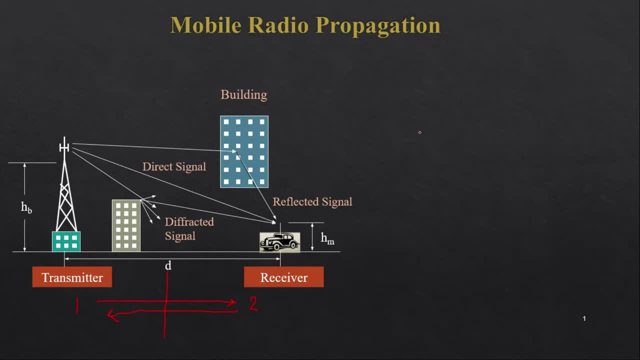 chapter we will discuss all these things. The first thing that we are going to learn in this chapter is large-scale propagation models. It predicts the mean signal strength for an arbitrary transmitter receiver separation distance, which are useful in estimating the radio coverage area of transmitter. 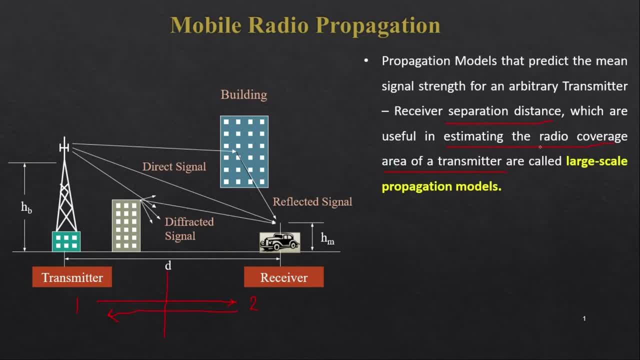 So this model are going to help us to identify the radio coverage area of transmitter, How much power should be transmitted by this transmitter to cover a particular area. Now the second types of models are small-scale or fading models. These are the propagation models that characterize the rapid 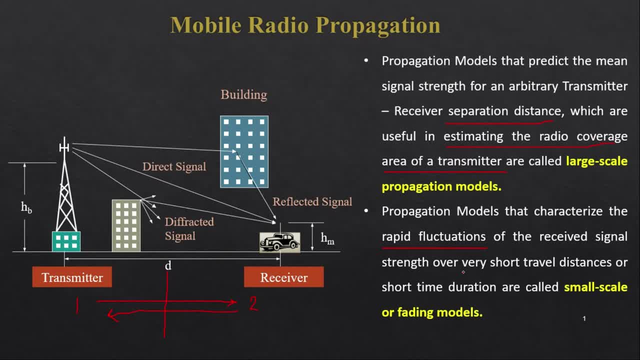 fluctuation of receive signal strength over a very short travel distance or short time duration. So, as we know, in a wireless system we have this mobile as moving object. So due to the rapid fluctuation or even a very small movement of this object, there may be some losses in a wireless 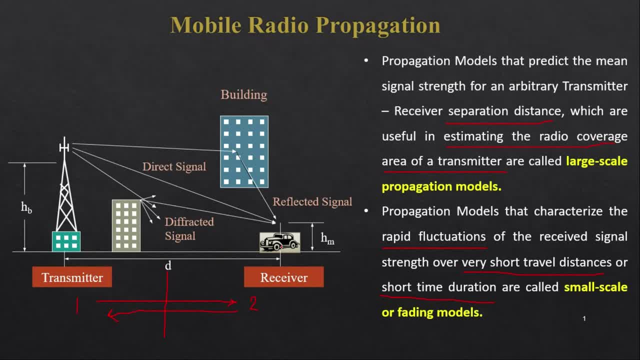 medium. So all these losses and all these predictions are related to the small-scale propagation models, or we can also call it as a fading models. So before we jump into all these things, we have to first understand what are the basic propagation mechanisms in a wireless medium. 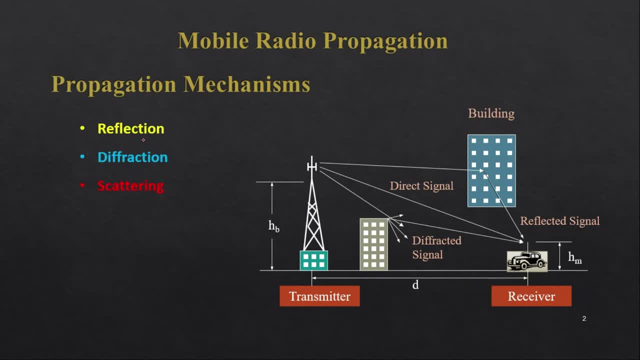 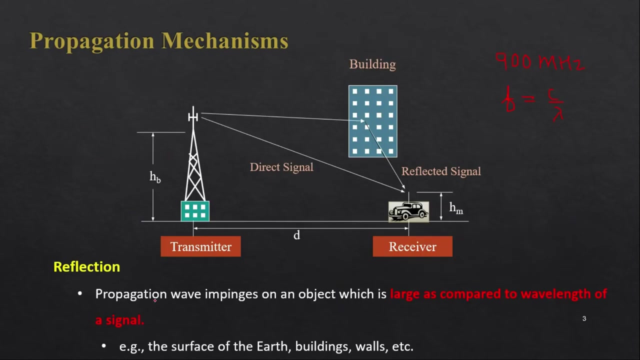 So there are three basic propagation mechanisms in a wireless medium. They are called as reflection, diffraction and scattering. We will see all these things one by one in this lecture. So now let us start with reflection. Reflection means propagation wave impinges on an object which 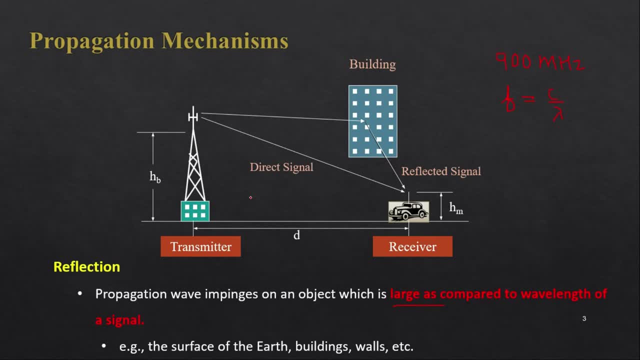 is large as compared to wavelength of a signal. Now how we will get wavelength of a signal? So let's say, in a wireless system we have a system that is operating on a 900 megahertz frequency. Now if we want to find out the wavelength, we can find it with the help of this equation, that is: 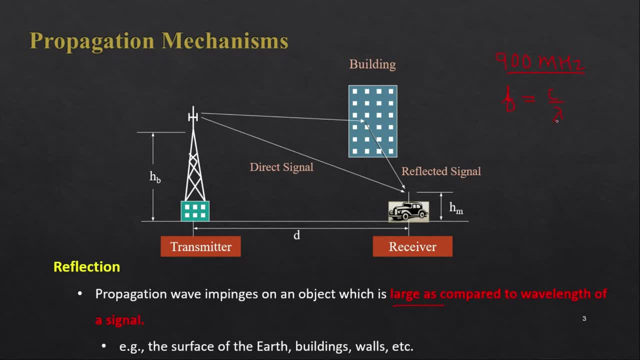 f equal to c by lambda. So frequency and wavelength are inversely proportional to each other. As we are going towards the higher frequency, we will find that the wavelength of a signal will become small. So now, whenever this wavelength, this particular wavelength, it can be in a few micrometer, or in, it can be in a millimeter. 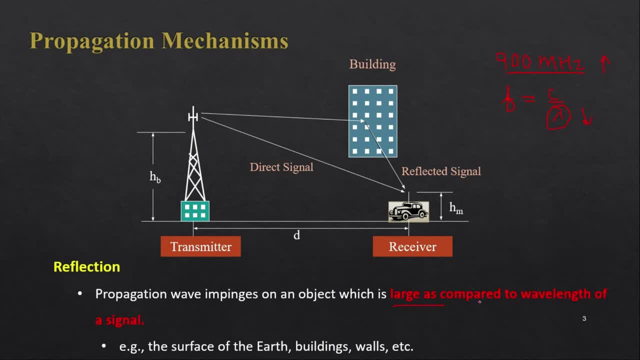 Ultimately, it will depend upon the frequency. If there is some object which is large as compared to wavelength of a signal, reflection will occur Here. the signal will travel from the transmitter and let's say, this building is the object, This building, and it will reflect back to this receiver. Why it will reflect back? because the 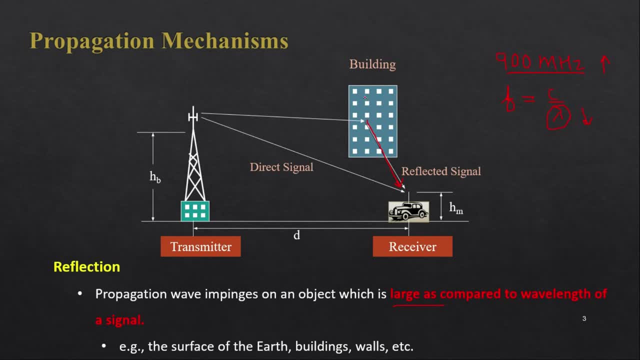 wavelength of this signal is very less compared to this particular object, building. You can also understand with the help of one tennis ball: if you will throw on a wall, it will reflect it back to you. So that is the example of reflection. In wireless system this kind of reflection will occur. 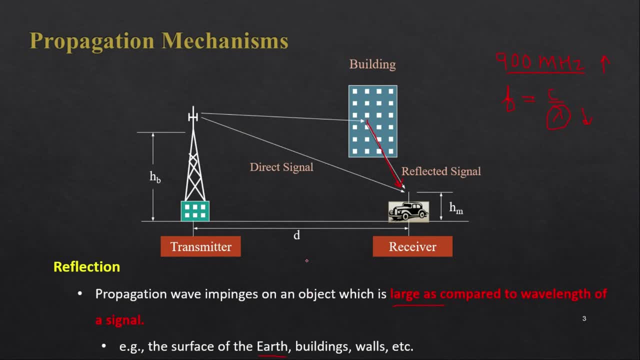 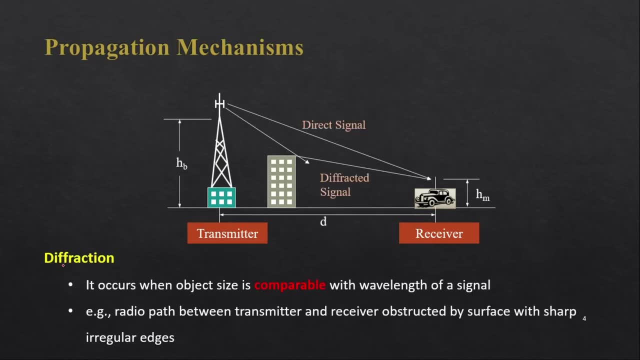 at the surface of a earth, which is very large compared to the wavelength of a signal, as well as buildings and walls and etc. Another propagation mechanism is diffraction, So it occurs when object size is comparable with the wavelength of a signal. That means the wavelength of a signal and object size are same. 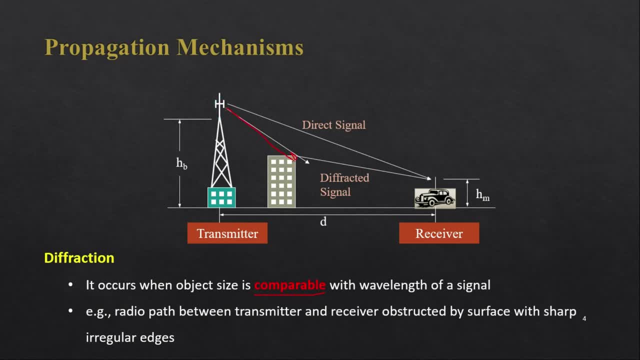 Now here the signal from transmitter will impinges on the edge of this particular building, which is visible. That means the wavelength size as well as the this object size, both are almost same. Then, instead of reflection, the signal will be diffracted, It will just change the path and 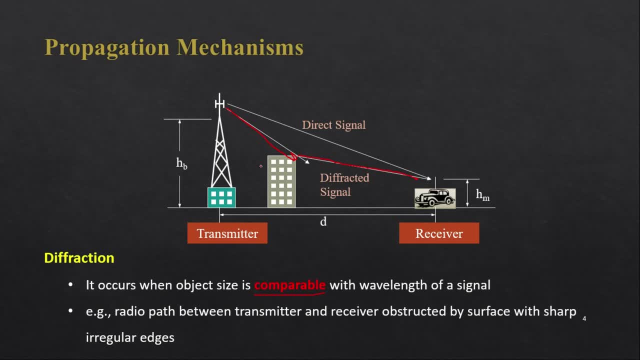 there will be a little bit losses over here, and this kind of scenario is called as a diffraction, The same thing you can understand. if you are throwing a ball on the edge, then it will be diffracted, Also due to the edge, instead of going towards, instead of going towards to the wicketkeeper, the